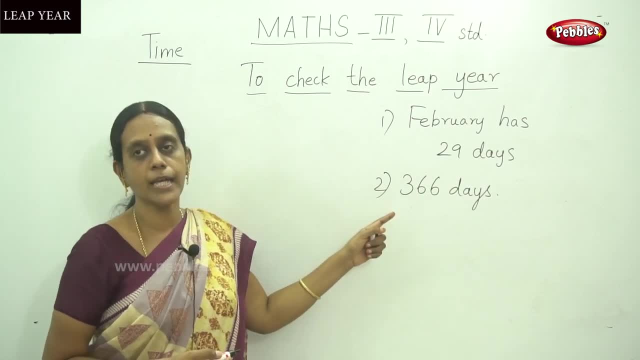 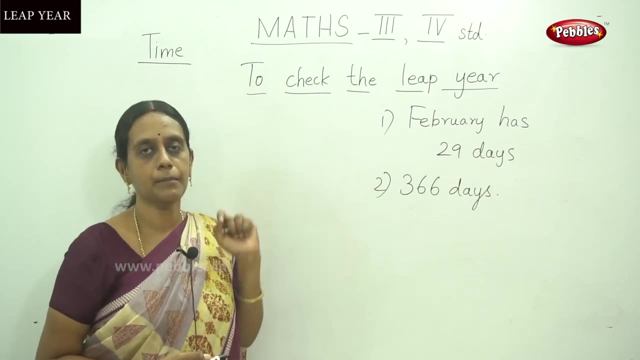 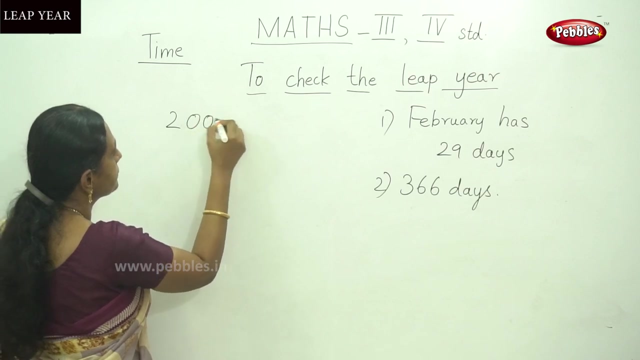 has 29 days and total number of days that is 366 days. Okay, and how to say it is a leap year and it is not a leap year that the digit that that means here, 2000.. Okay, Okay, this is the first year, and 2000, that is 18 and 2000.. 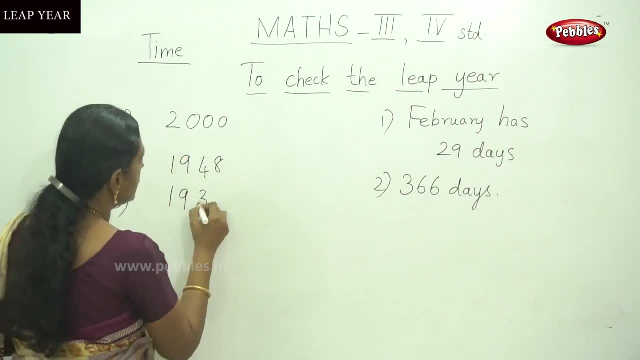 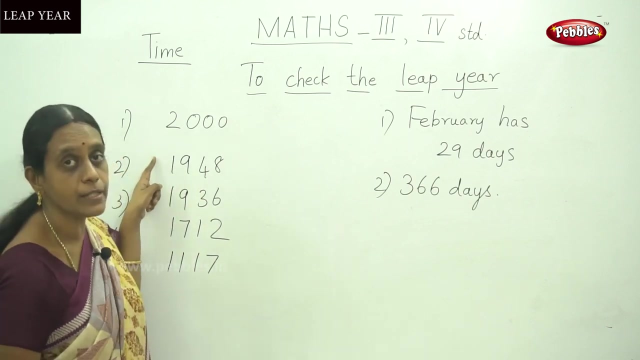 1948. Okay, And Okay it is here. here are the persons. or here that is 2000, 1948, 1936. Okay, 1712, that is, and 1117, that is 1117.. So here that is said. that number is divisible by. so you have to check the. 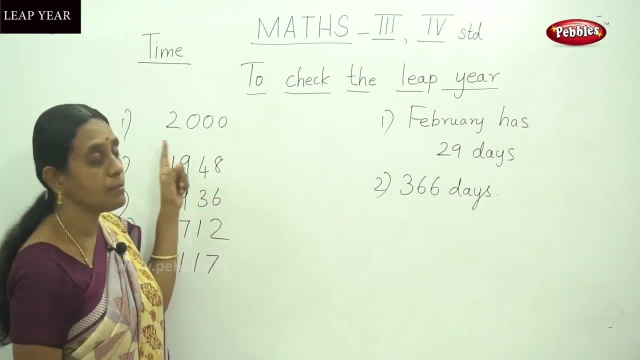 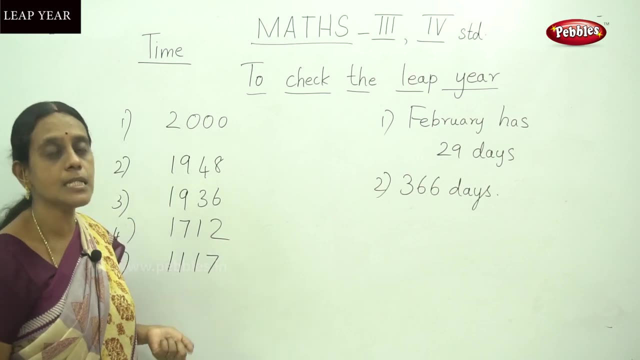 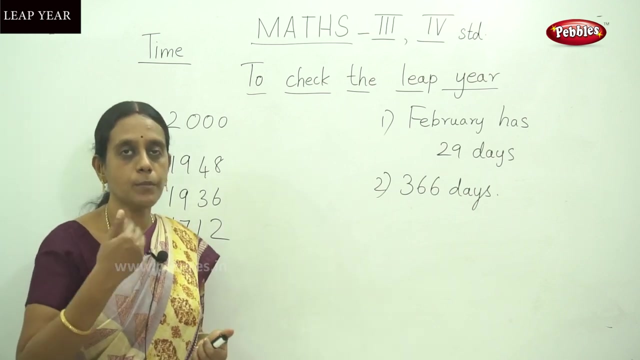 number, whether the number is divisible by the number or not. So here here the number is divisible by 4 or not. ok, for divisibility of 4. we have discussed the rule in our test in divisibility heading. we have already discussed the divisibility of so many. 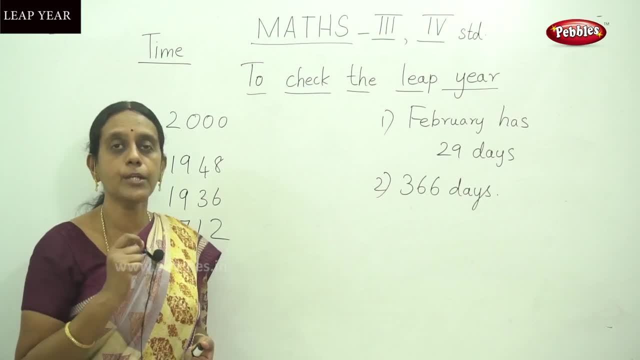 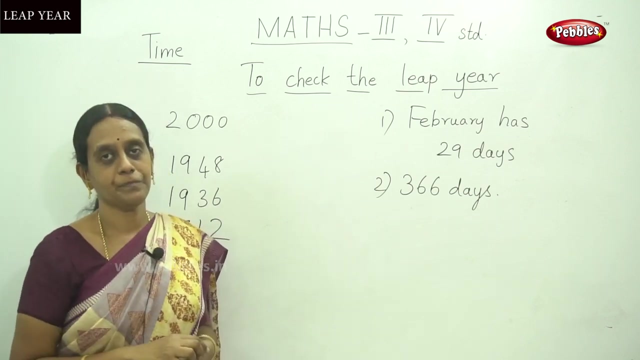 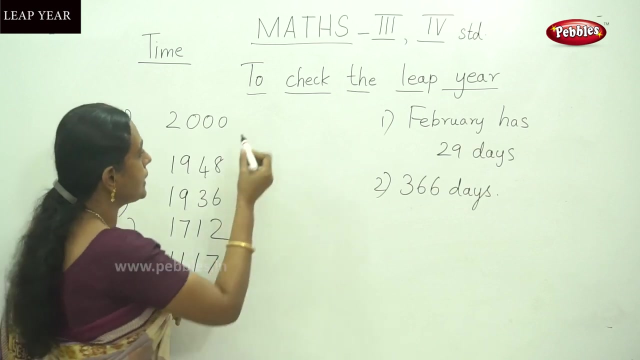 numbers that we have. we should recap the divisibility rule of 4. that means the last two digits are 0 and the last two digits are the divisible by 4. the number is divisible by 4. ok, do you understand that for this you have to check the divisibility of 4? all these number. 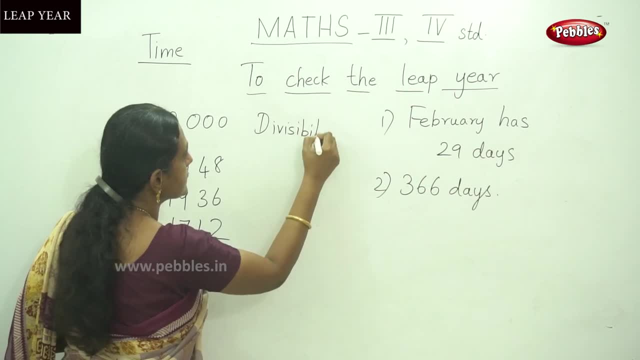 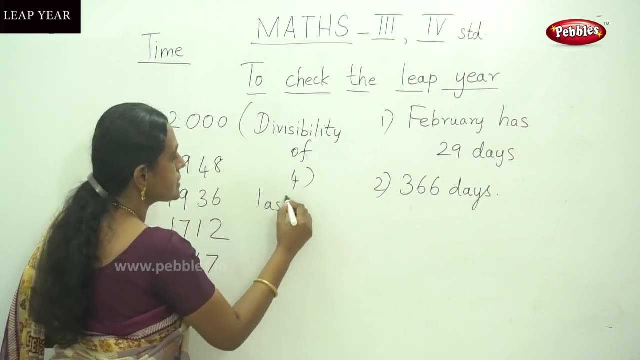 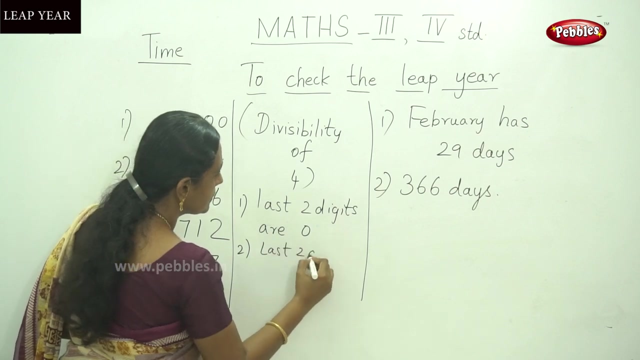 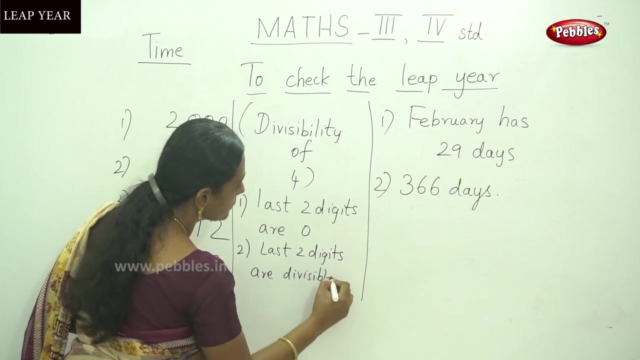 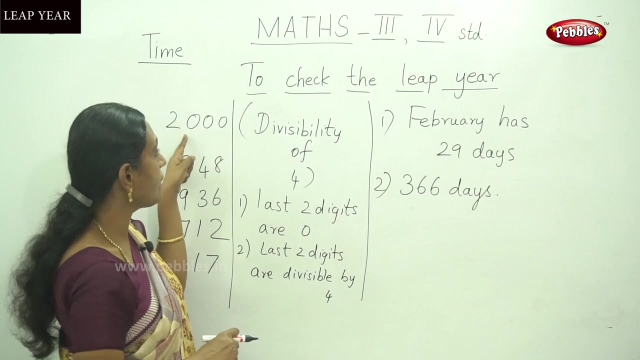 you have to check that is divisibility of 4. that is, divisibility of 4 means last two digits are 0. are. last two digits are 0. okay, and last two digits are. that is divisible by 4.. This is a divisibility rule for 4.. By check out these rule, you have to say this number, whether it. 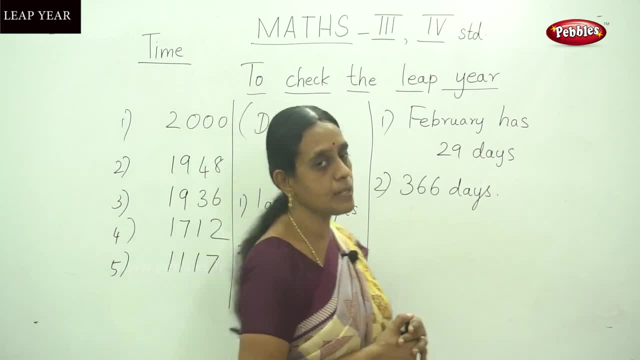 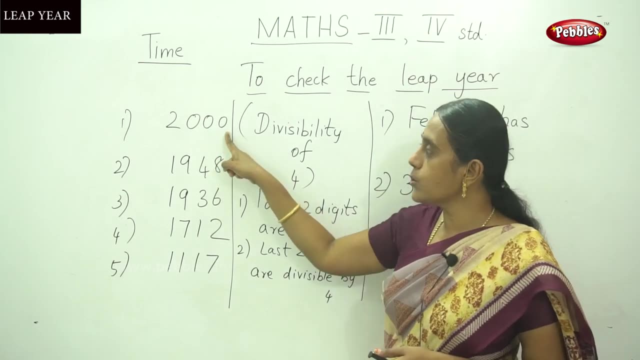 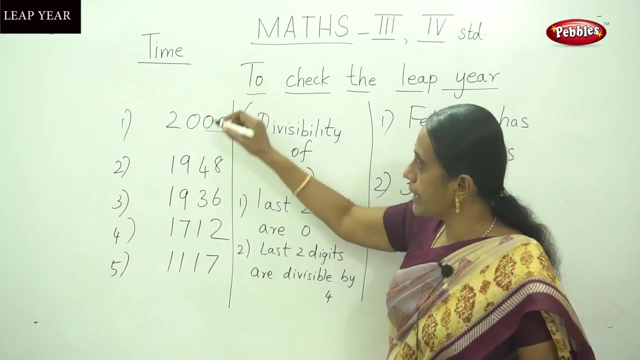 is divisible by 4 or not. Suppose this number is divisible by 4 this year, this number is a leap year. okay, That means here last two digits are 0. So hence improve the divisibility rule. So this is a leap year. okay, 2000 is a leap year, and here the last two digit that. 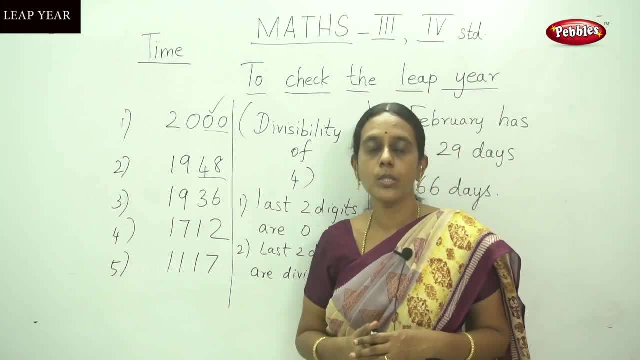 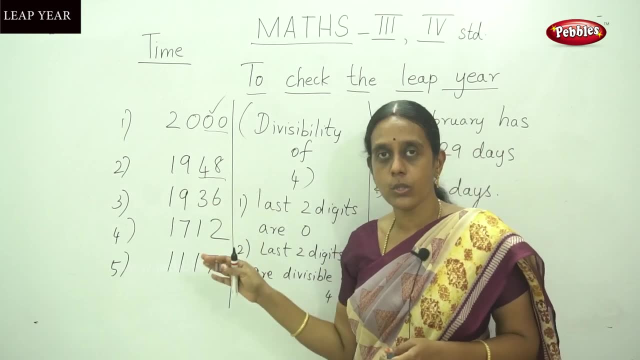 is 48.. 48 is divisible by 4, because it is a multiple of 4, that is 12, 4s are 48. So this is a leap year, Hence 1948, also leap year. So that year, that February month has. 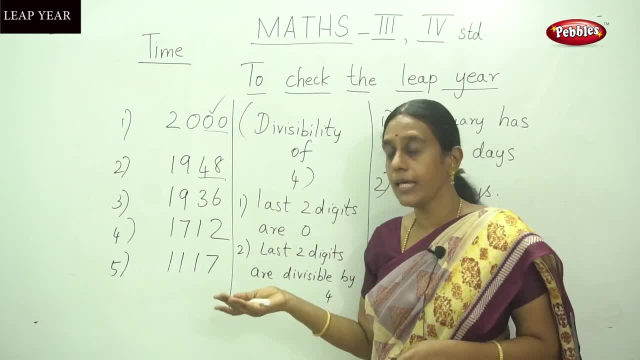 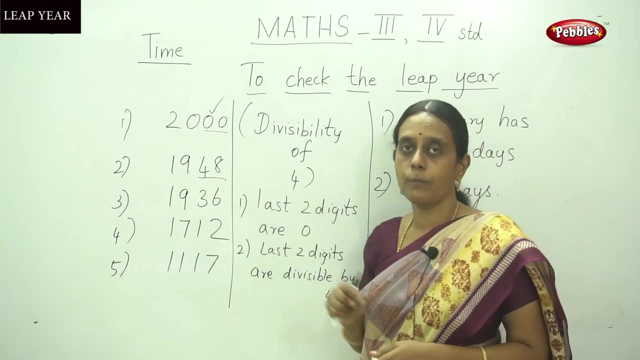 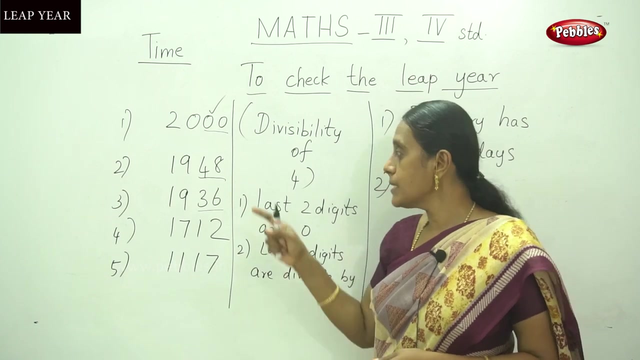 29 days without division. we can say this: is it is a leap year or not? by proving this 4 divisibility of 4 rule: okay And 1936.. So by checking this last two digit number, that means that is divisible by 4: okay, 9. 4s are 36.. 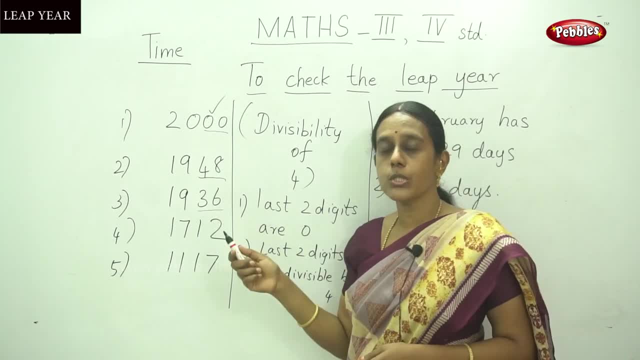 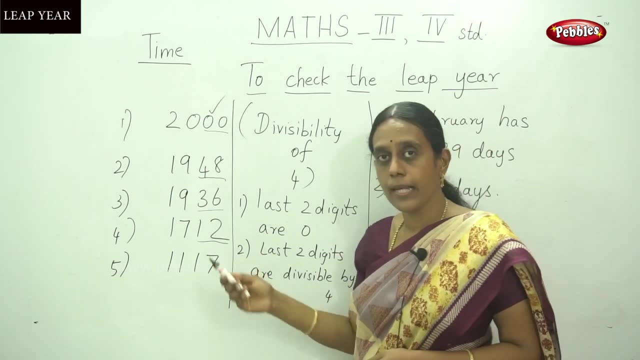 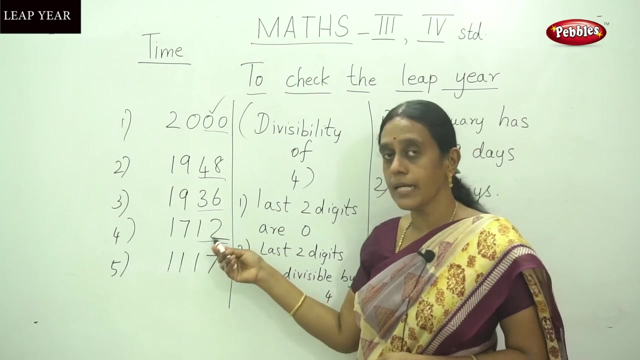 Hence, this year is a leap year, and that year also, that February month has 29 days, okay, And here check out this last two digit, that is 12. okay, This is also a divisible by 4, that is 3, 4s are 12.. Hence, this year is a leap year, okay, And last, that is two digit. 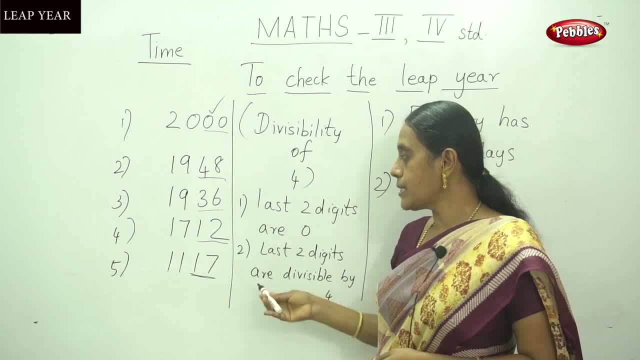 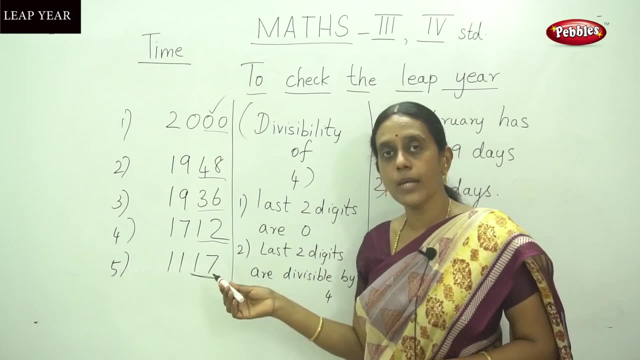 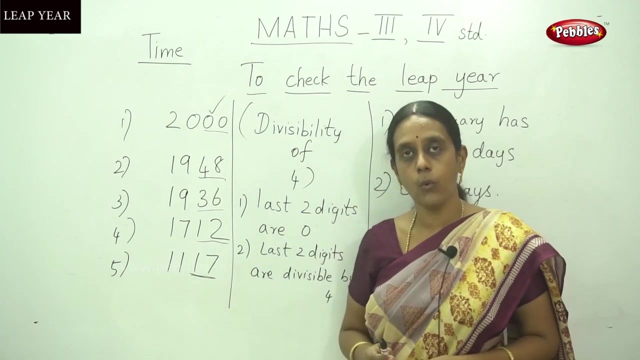 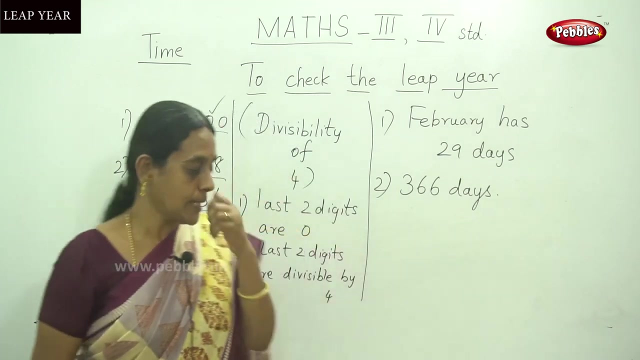 that is 17.. It does not prove these, both these rule, because the last two digits does not have zeros, Okay, And that number 17, that is 17, that should not be divisible by 4. It is not a multiple of 4. So this is not a leap year. So, among these all 5 years, that is 2000. okay, All these. 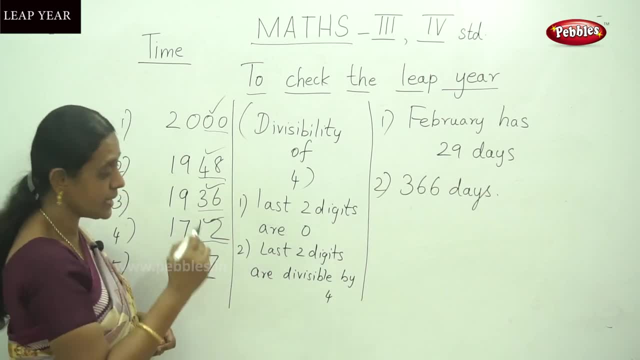 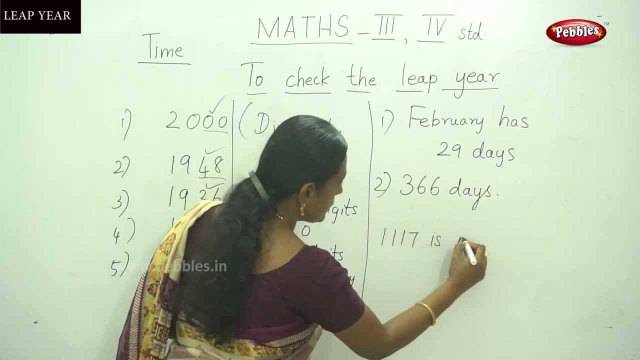 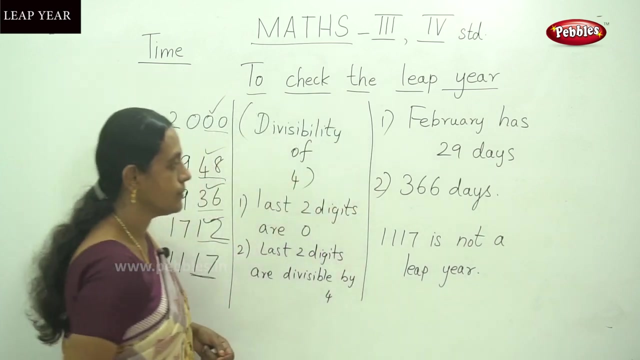 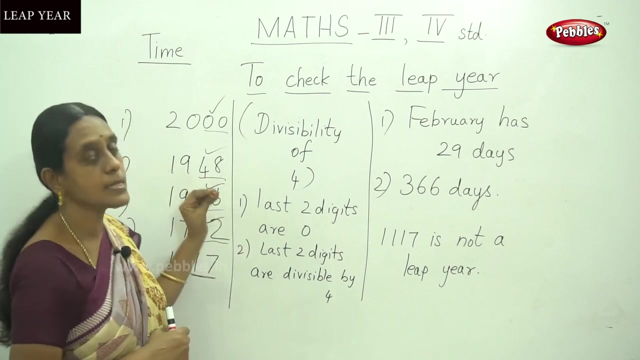